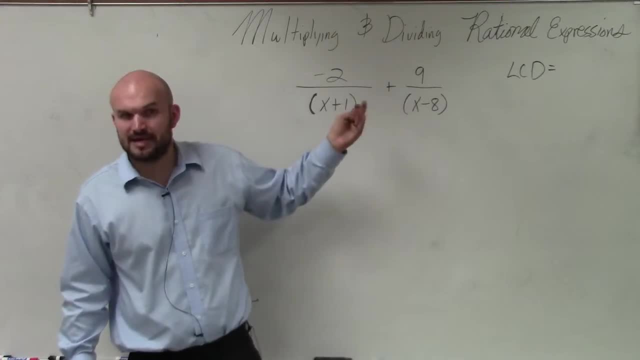 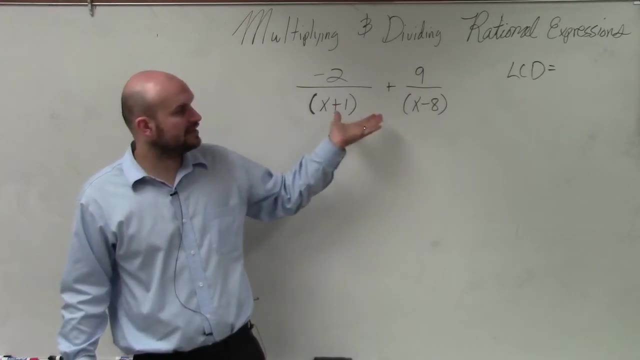 that, more than likely, is always going to be case, unless they're already in the same. But so basically what I would do here, since it's not very apparent on what they share, the only the common denominator that they're both going to share is going to be their product, which would be x plus. 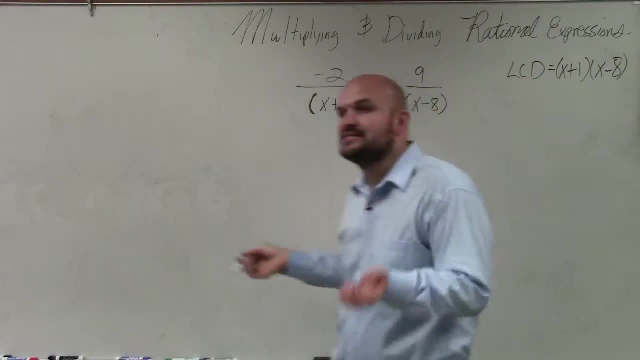 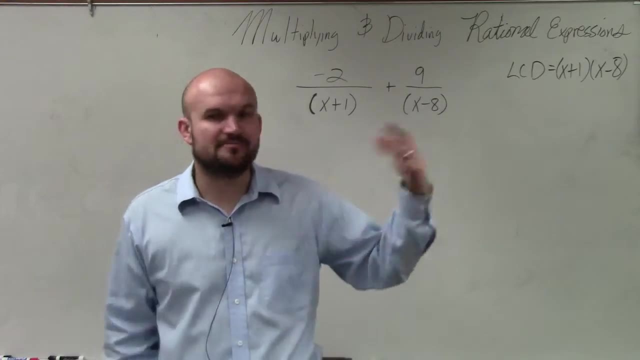 1 times x minus 8.. So the LCD is simply their product, just like the LCD was 21, 3 times 7.. Okay, Again, it's not always going to be that case, but very often it will, And now we're going to do an. 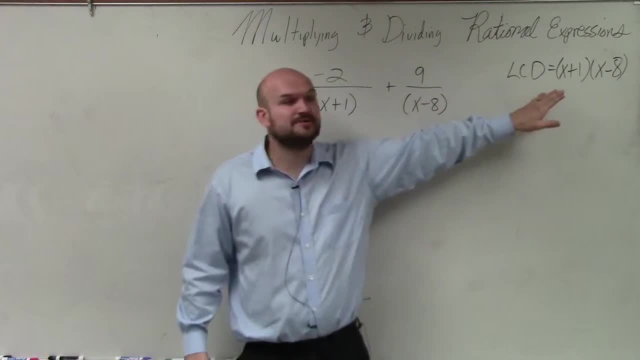 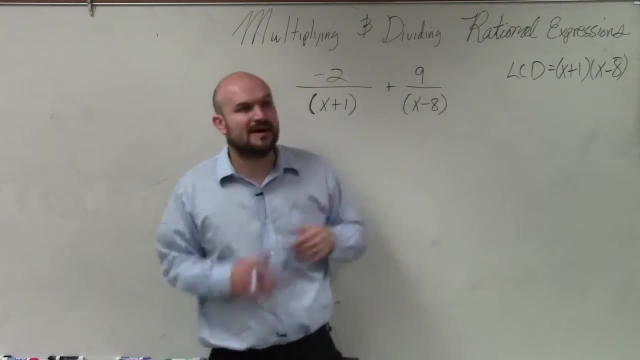 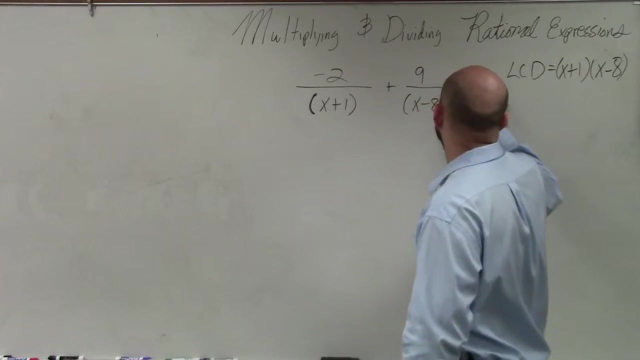 example, next time where it won't. So if here's my LCD now, I need to determine how do I get x minus 8 to be x plus 1 times x minus 8.. What would I need to multiply x minus 8 by x plus 1.. And whatever? 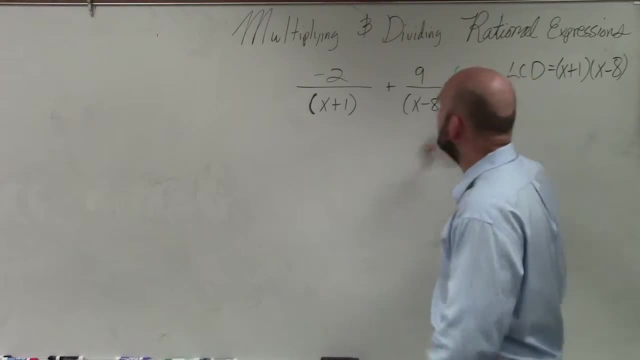 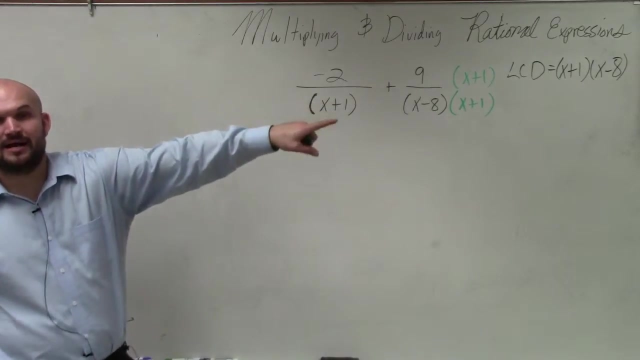 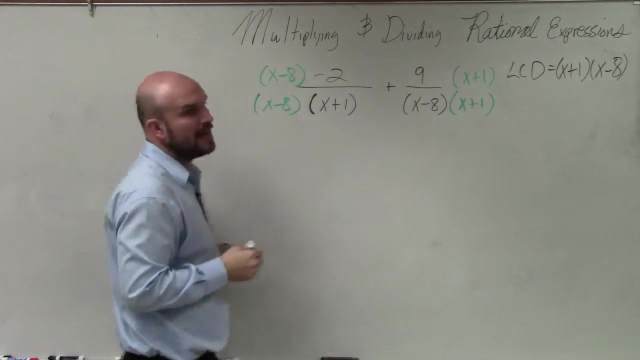 I do in the denominator, I have to do in the numerator. Over here I have x plus 1 in my denominator. To again determine, to get this to my common denominator, I need to multiply it by x minus 8.. So now what you guys can see is: now I need to simplify my numerators. So to simplify my 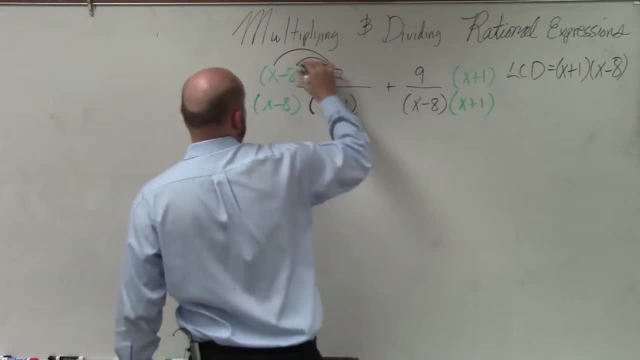 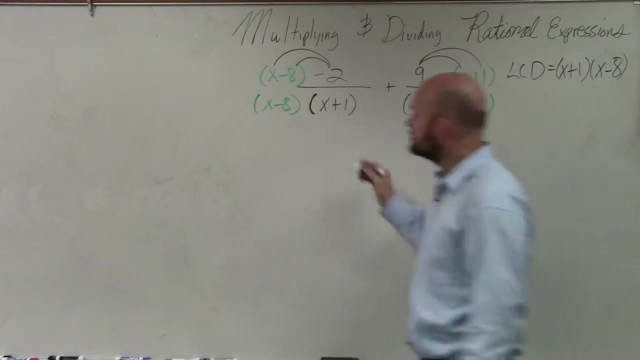 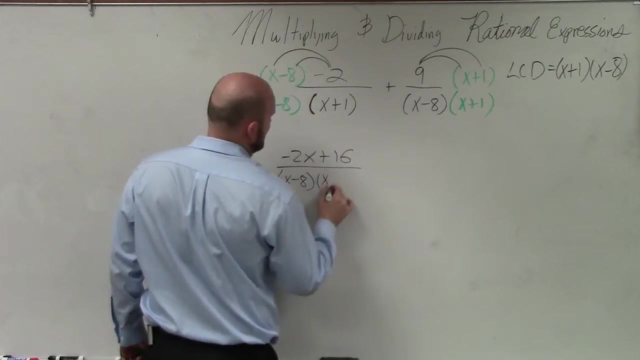 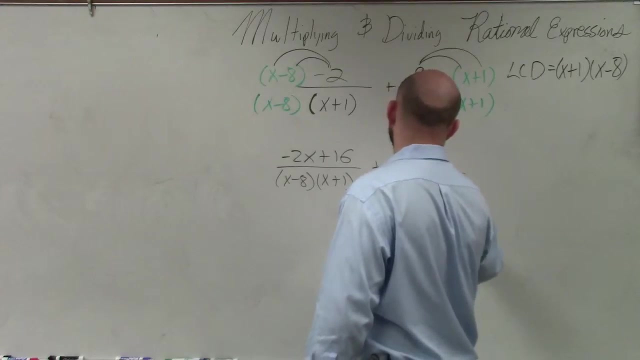 numerators, I need to apply just derivative property. Okay, Now, you could multiply this out, but I'm just going to leave this as a product down below. So what I have here then is negative 2x plus positive 16.. All over x minus 8 times x plus 1 plus 9x plus 9. all over x minus 8 times x plus 1.. 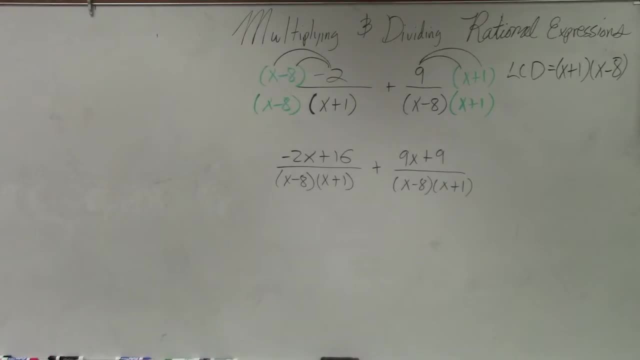 Okay. So what I'd like you guys to see now is: you see that we have now two fractions with the same denominator. So when we have two fractions with the same denominator, we just combine the terms in the numerator. So I'm just going to combine 9x and negative 2x. 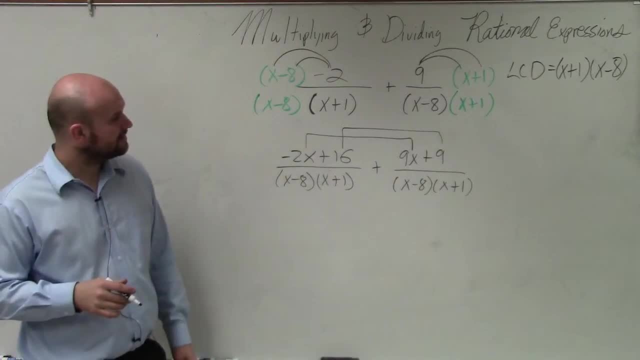 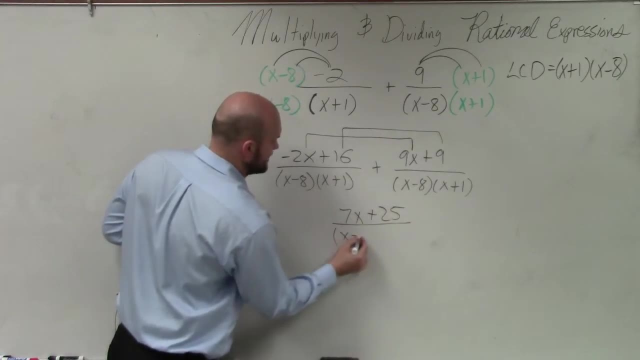 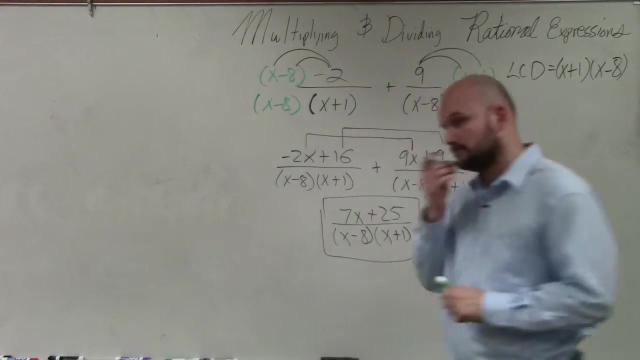 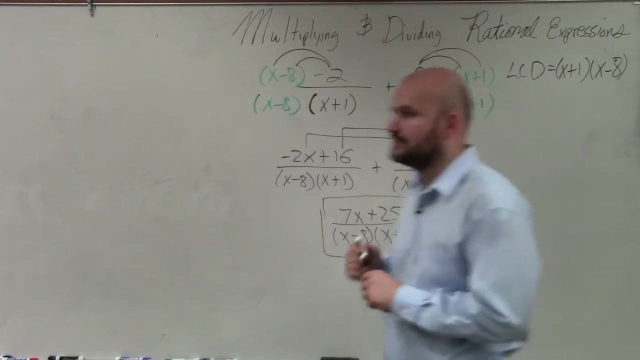 16. and 9.. Okay, So this becomes 7x plus 25, all over x minus 8 times x plus 1.. Yeah, I mean you could multiply through the denominator if you want to. I just prefer a lot of times. 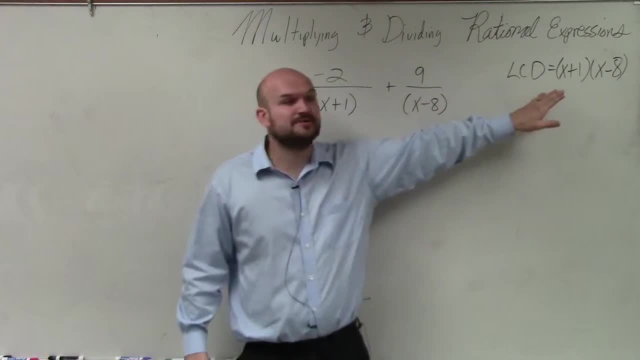 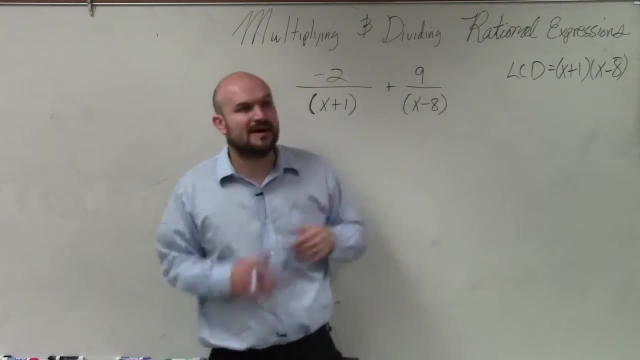 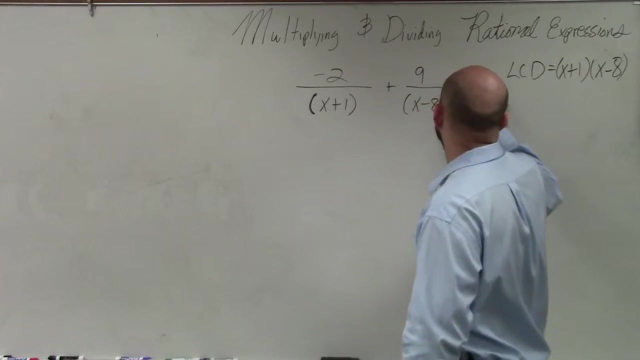 example, next time where it won't. So if here's my LCD now, I need to determine how do I get x minus 8 to be x plus 1 times x minus 8.. What would I need to multiply x minus 8 by x plus 1.. And whatever? 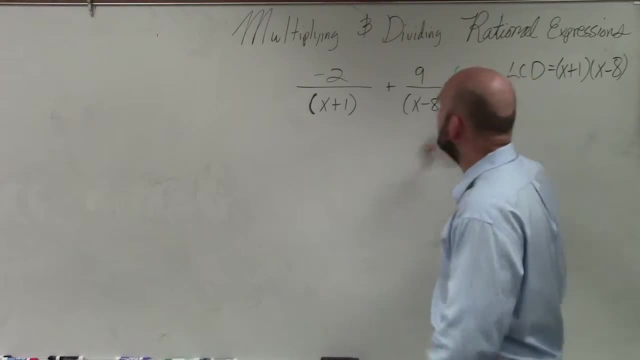 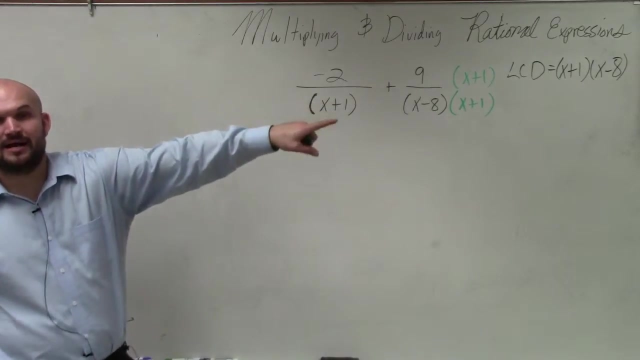 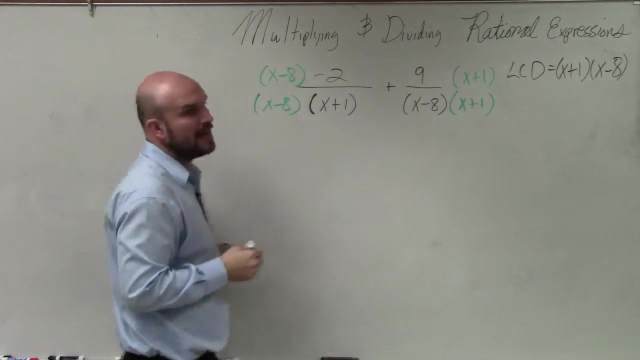 I do in the denominator, I have to do in the numerator. Over here I have x plus 1 in my denominator. To again determine, to get this to my common denominator, I need to multiply it by x minus 8.. So now what you guys can see is: now I need to simplify my numerators. So to simplify my 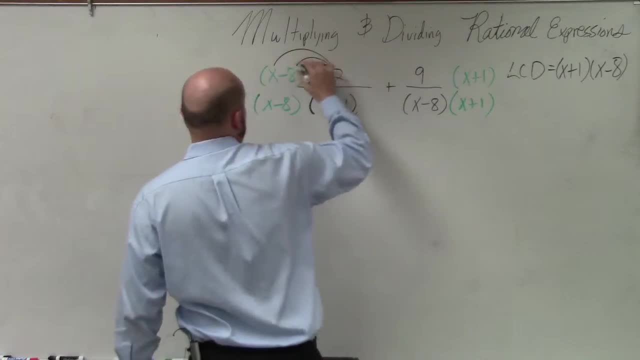 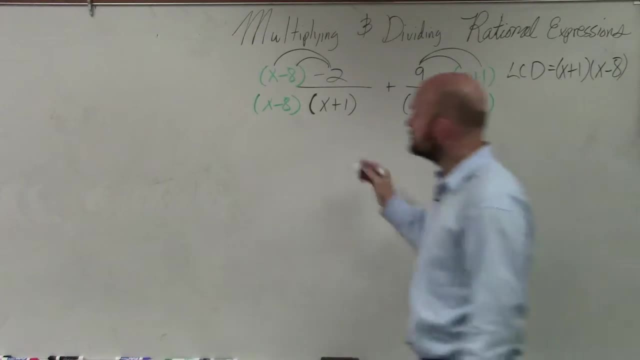 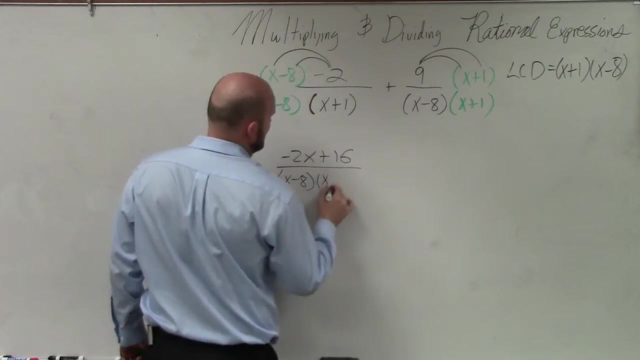 numerators, I need to apply just derivative property. Okay, Now, you could multiply this out, but I'm just going to leave this as a product down below. So what I have here then is negative 2x plus positive 16.. All over x minus 8 times x plus 1.. 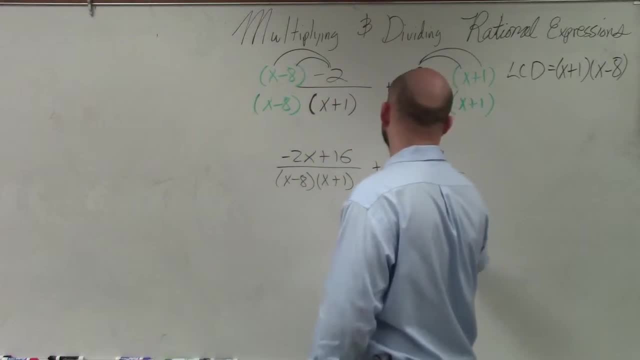 Plus 9x plus 9.. All over x minus 8 times x plus 1.. Okay, So what I would like you guys to see now is: you see that we have now 2 fractions with the same denominator. So when we have 2 fractions with the same denominator, we just combine. 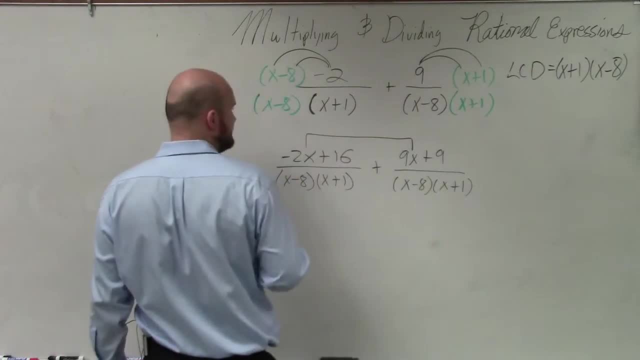 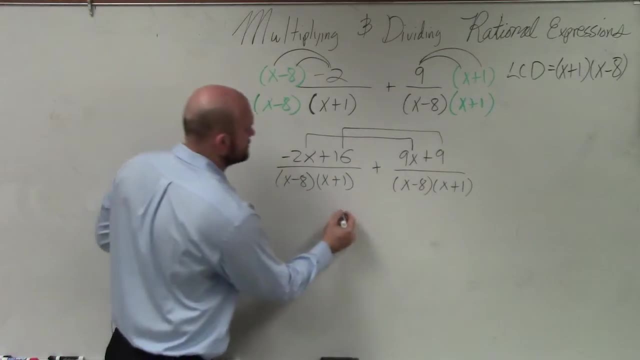 the terms in the numerator. So I'm just going to combine 9x and negative 2x, 16. 16, and 9. So this becomes 7x plus 25,, all over x minus 8 times x plus 1.. 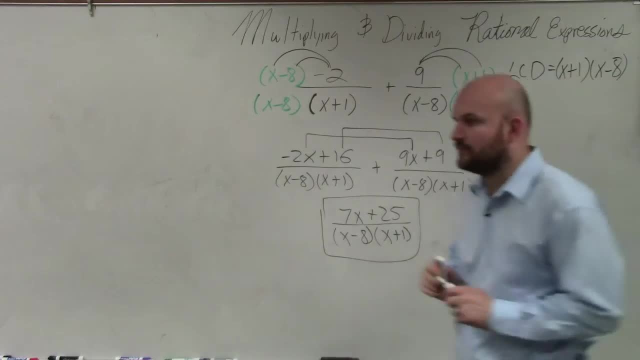 Yeah, I mean you could multiply through the denominator if you want to. I just prefer a lot of times just to leave it and multiply it out. OK, any questions? 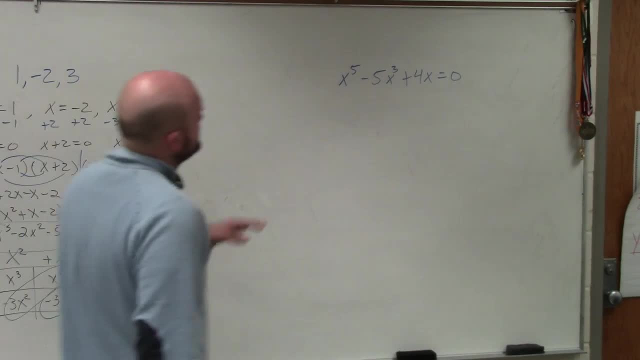 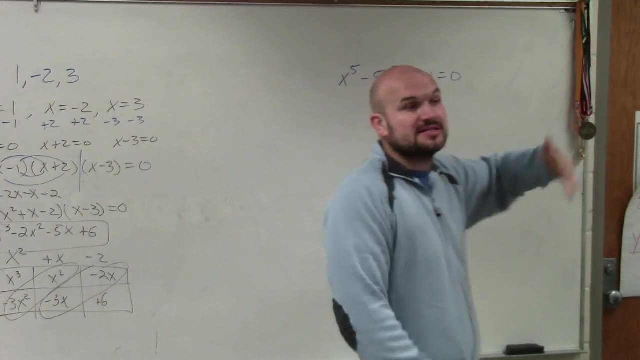 So the last one here states: ladies and gentlemen, we have x squared x to the 5th, minus 5x cubed plus 4x equals 0.. So what we did last class was I showed you guys some factoring techniques. 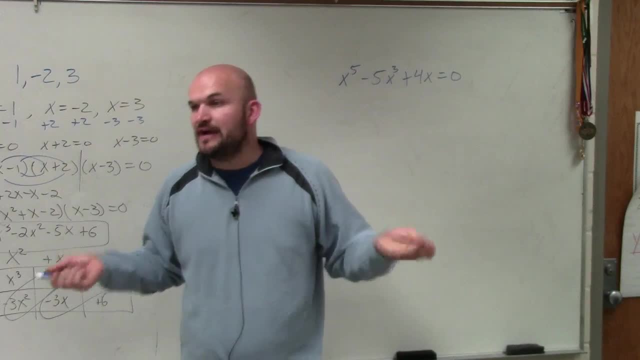 The first important thing, guys, is we always want to see: can we factor out a GCF, Can we factor out a common factor? And you look at all these and you say, yeah, they share something. What do they share, though? 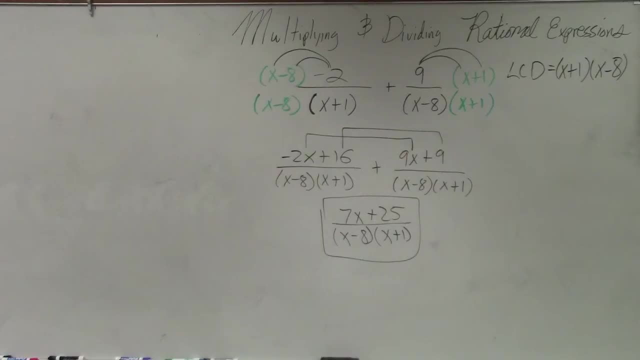 just to leave it and multiply it out. Okay, Any questions?